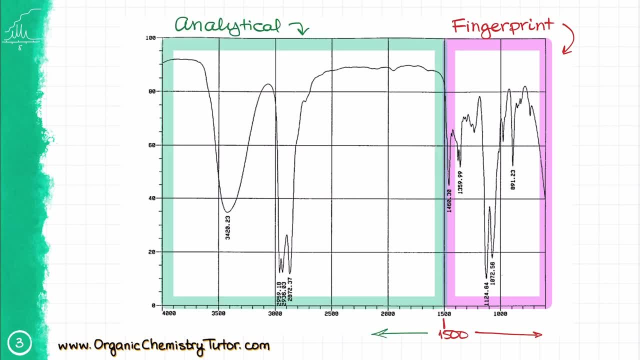 reciprocal centimeters and we have the analytical region above 1500 reciprocal centimeters. Anything we care about is going to be in the analytical region right over here. The fingerprint region will only be useful for you if you are trying to identify your molecule by comparing. 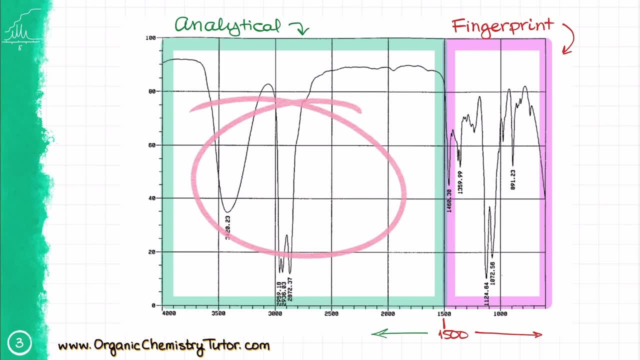 it to a known sample. The fingerprint region works well. like a fingerprint, It's pretty much unique for each molecule. However, it is nightmarishly difficult to interpret unless you really know what you're looking for. So we'll leave this to the pros and focus on the 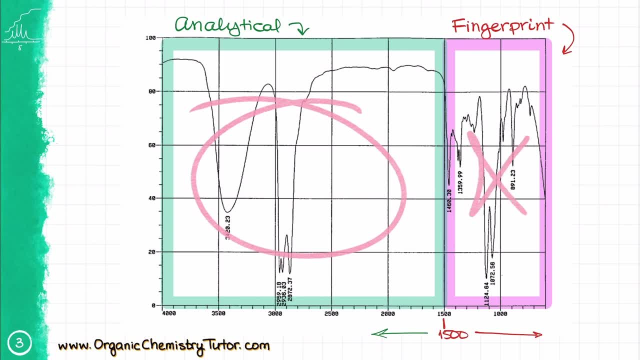 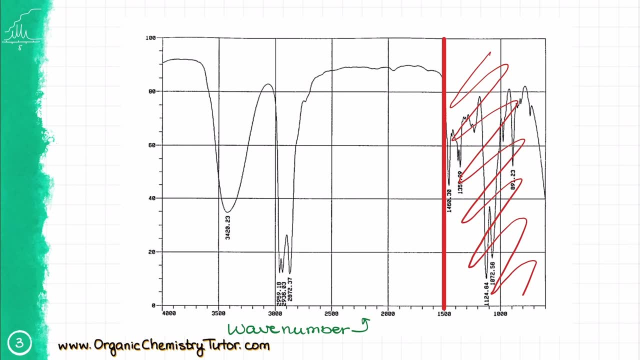 analytical region of the spectrum. So the fingerprint region is something that we don't really care about. So what type of information are we going to get from the analytical region? First of all, the wave number, which is these numbers over here. 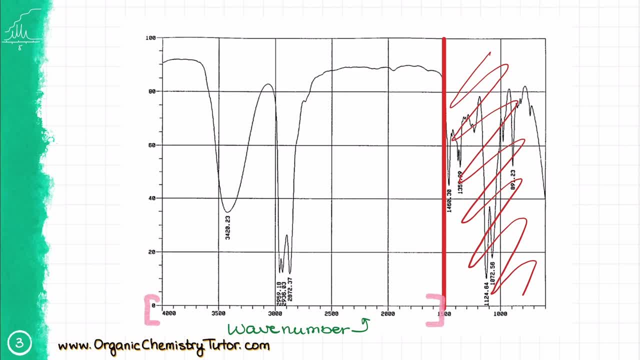 It's typically expressed in reciprocal centimeters and it's related to the vibrational frequency, which is directly proportional to the energy with which our bonds are vibrating. So the higher the wave number, the higher the energy with which the bond vibrates. 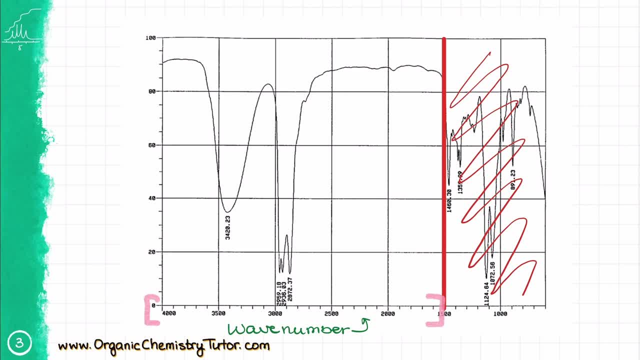 So, for instance, on this spectrum I have a couple of signals: One at about 3400 reciprocal centimeters and another one at around 2850-2950.. In addition to the wave number, I have a couple of signals that are similar to the wave number but they're a little bit different. So the 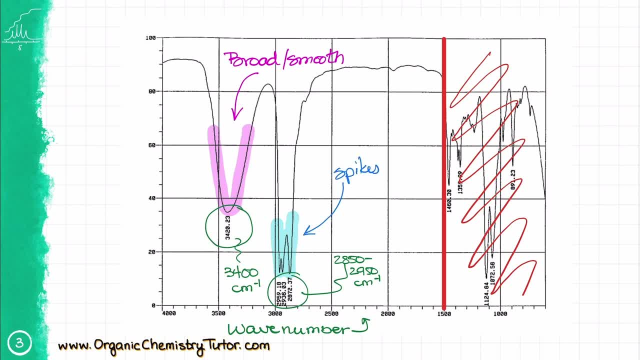 wave number will also look at the signal's shape, So like, for instance, this signal is broad and smooth, while this one is very spiky. And finally, the least bit of information for us is going to be the signal's strengths, which can be strong if it dips down below. 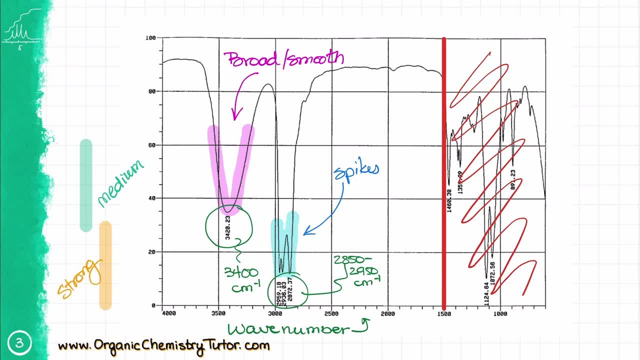 30% transmittance. medium if it is somewhere in the middle of the transmittance scale. and weak if the signal is higher than 70 or so. important piece of information, as the strength will depend on how the spectrum was obtained and what exactly the molecule is. all about The same molecule. 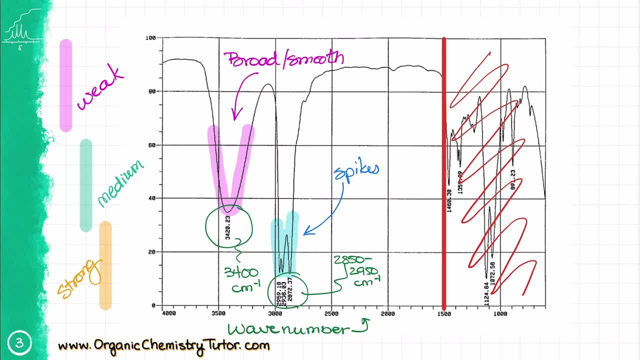 can have differently looking signals in terms of their strength, depending if the spectrum was, let's say, obtained from the thin film or potassium bromide, mold or neutral mix, etc. What will be the same, though, is the position of the signal and its shape, So once you get your wave numbers and the shape, you can match. 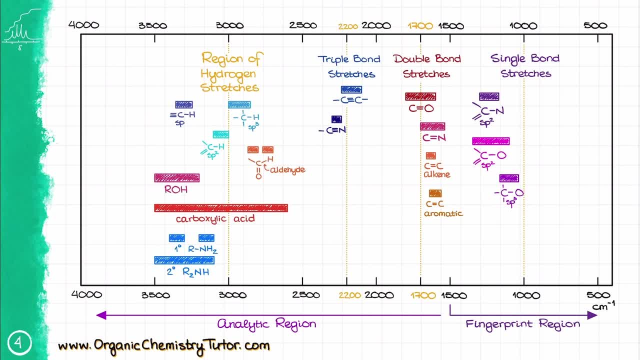 those to the reference table. So, for instance, here is the reference table I give to my students. This one visually represents the position of the signals in the spectrum. so it's kind of easy to match what you're seeing in the spectrum to what we have on the table. If you like this one, you can always download it from. 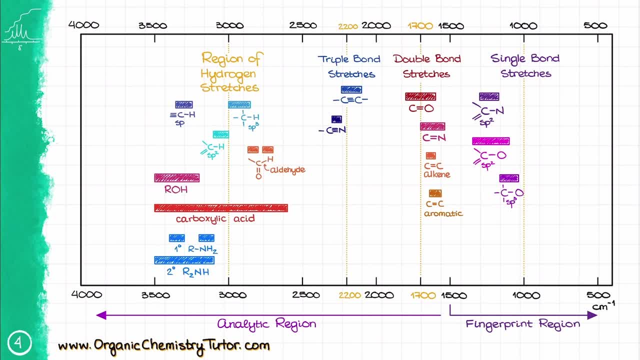 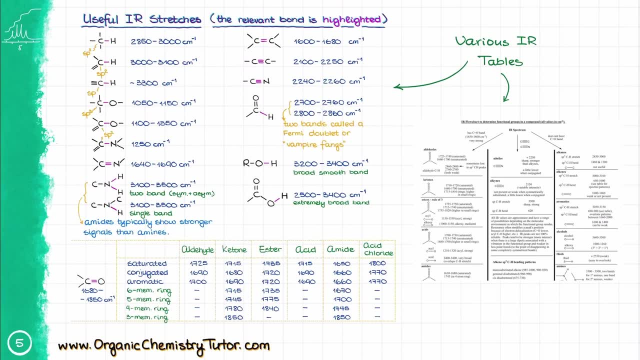 Organic Chemistry Tutor dot com, but I'm pretty sure your textbook has something similar to that- Well, maybe not that pretty- Or The reference table. reference table can be given to you in the form of an actual table. I suggest you choose whichever table works for you and learn how to use it efficiently. Some people like the 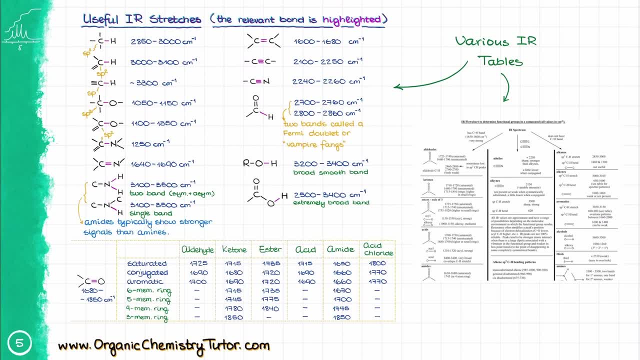 visual one, some people like the table one. whatever works will work for you. doesn't matter which table you choose. But whichever table you choose, you got to learn how to use it properly. I'm not going to tell you to memorize most common numbers, but I'm going 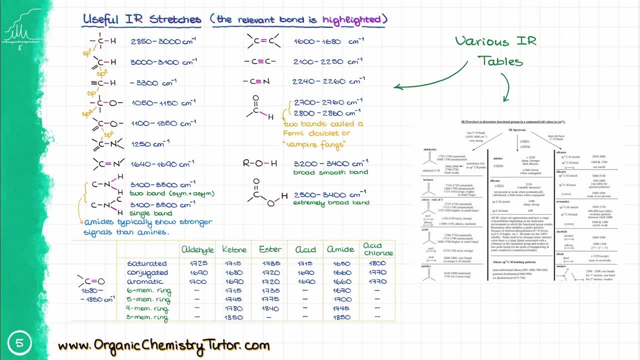 to tell you to memorize most common numbers. Here's the deal, though. Even if you are efficient at finding your reference numbers and know your IR table like the back of your hand, it is still going to take a few seconds here and a few seconds there to compare those numbers. 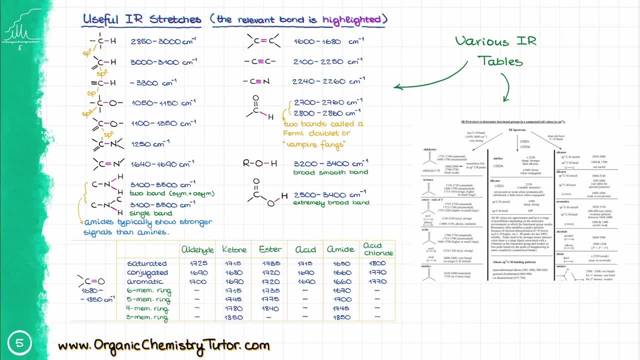 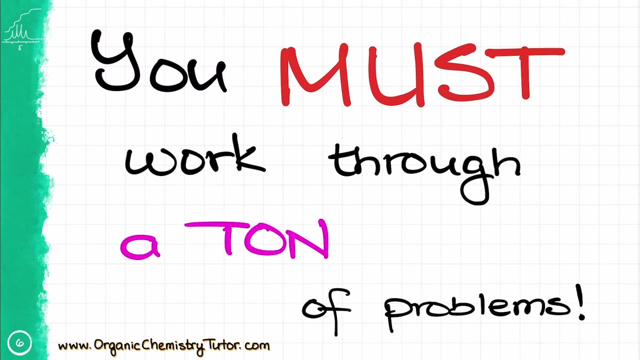 And those seconds will add up very quickly on the test. The good news, though, is that you'll memorize those numbers anyways if you do enough problems, Which brings me to the most important point of this video. You must work through a ton of problems. That part is not optional- If you want to be able. 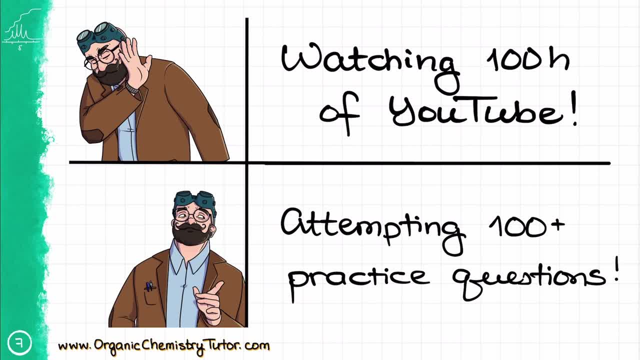 to solve these problems you need to practice, And when I say practice, I mean attempt to solve as many problems as you can, Not watch somebody solving them. Recognizing how someone solved a puzzle and solving a puzzle yourself are two huge differences. But enough of me. 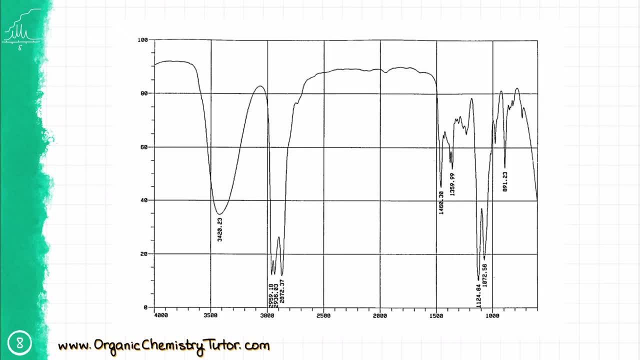 ranting here, Let's get back to our IR. When I solve my IR spectra I always look at the spectrum from left to right. The area around 3500 rc typically houses the OH and NH groups. So, for instance, in this case we 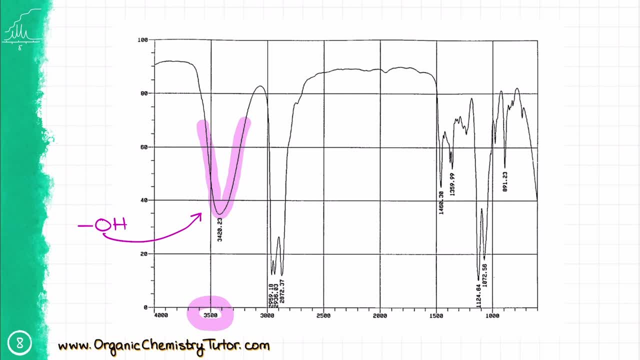 have a broad and smooth signal, which is the OH group. But how do I know it's not the NH, you might ask? Well, that's where the shape of the signals come into play. The OH is typically broad and smooth, While the NH is typically wide and smooth, When the OH is typically 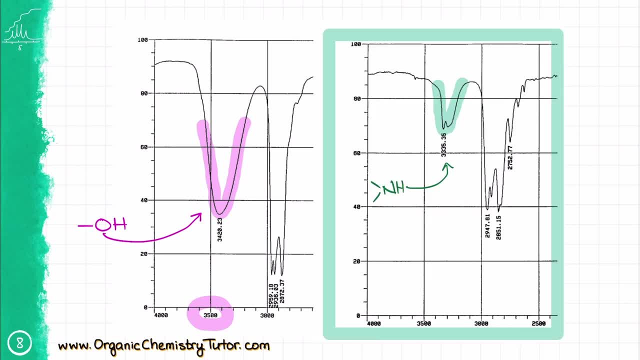 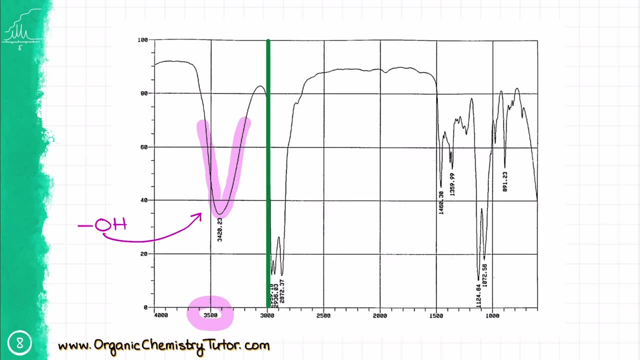 weaker and sharper. So here is the NH signal and how it looks like for the comparison. See, it's much weaker and much sharper than the OH group. Then we have this 3000 line. This is a very important line in the IR because this is where you normally see your carbon hydrogen stretches. 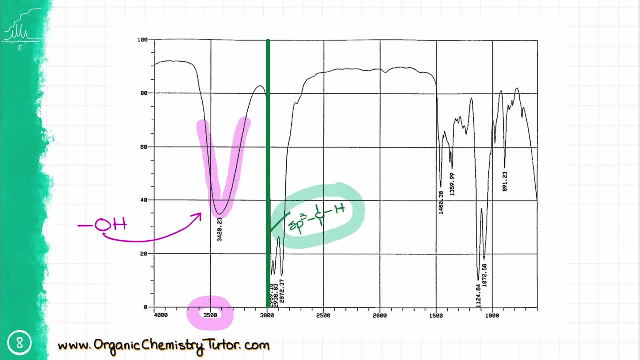 Signals leaning onto the 3000 from the right, or in other words signals that are hair under 3000, so about 2950 or so, are the regular sp3 hybridized carbon hydrogen stretches. You should see those signals for the majority of your compounds. Signals leaning onto your 3000 from 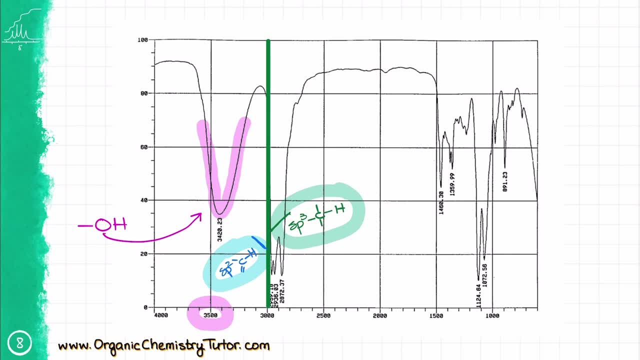 the left side, or in other words, signals that are just a little bit over 3000, like 3050,. those are sp2- hybridized carbon hydrogen stretches. So you'll expect to see those guys if you have double bonds in your molecule and those double bonds have hydrogens on them. 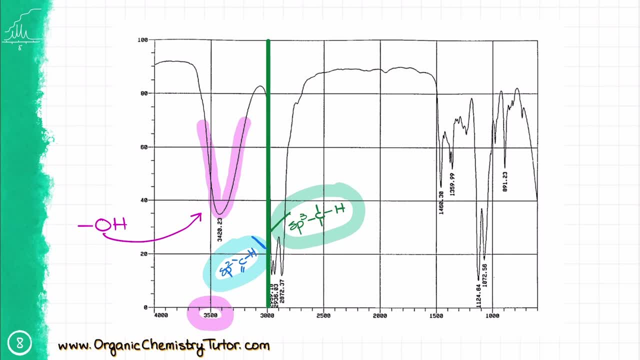 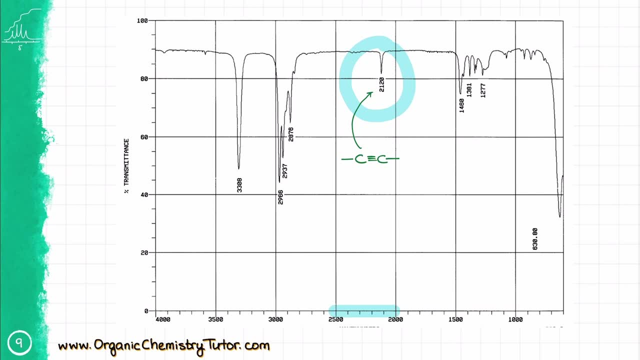 This molecule doesn't have any, so we are not seeing anything there. The next important region we are going to look at is going to be around 2500 to 2000 reciprocal centimeters. This is where the triple bonds leave. Those signals are typically pretty weak and can sometimes completely disappear. 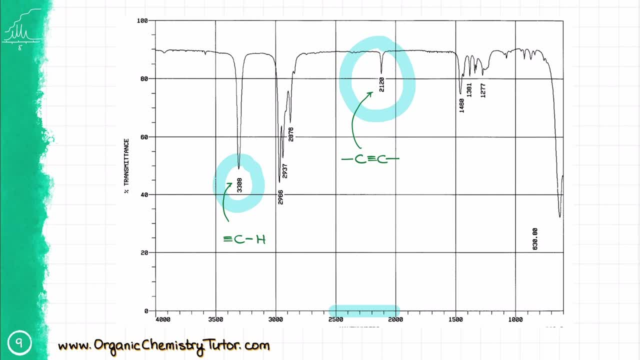 But if it is a terminal triple bond like what we have here, we are going to have a sharp spike at almost exactly 3300 centimeters, which is the sp- hybridized carbon. It's a somewhat rare signal, since we are only going to see it for the terminal triple bond. 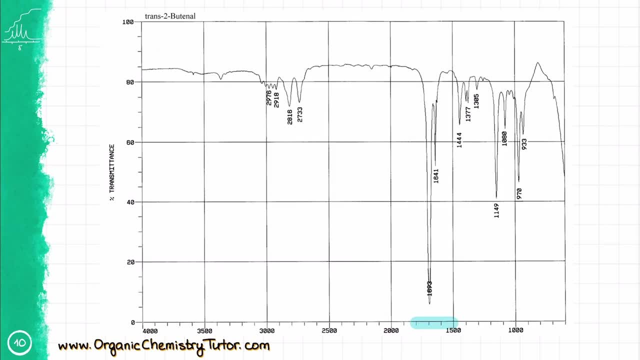 but nonetheless you should be familiar with this signal. The next important region is the 1800 to 1500 centimeters, which is where we have various double bonds. For instance, in this case, I have a CO double bond at roughly 1700, and I also have a CC double bond at about 1650.. These are, of course, 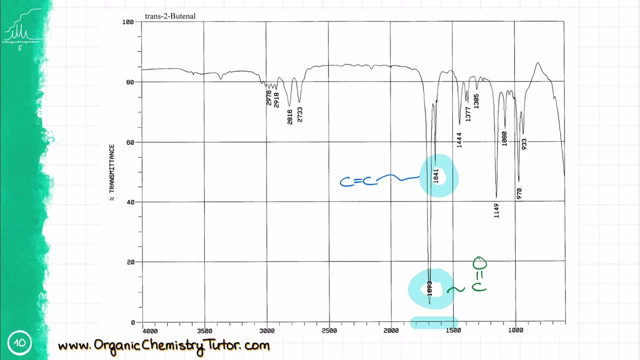 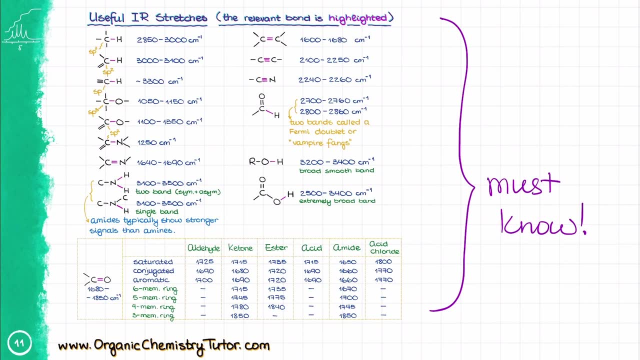 the dominant functional groups you'll be looking at in your molecule. There are many other ones that can potentially pop up in the analytical region and with practice you will learn to recognize those as well. With time and practice, you'll learn to recognize all of these functional groups. 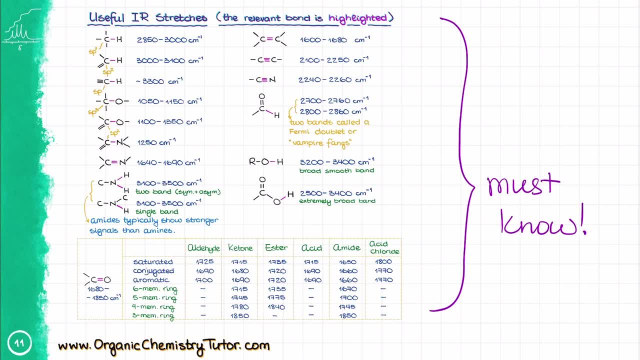 and will memorize most of these numbers as well. You'll also be able to recognize some signals in the fingerprint region. but unless you are comfortable with the analytical region first, which is above 1500 reciprocal centimeters, don't even poke your nose into the fingerprint. 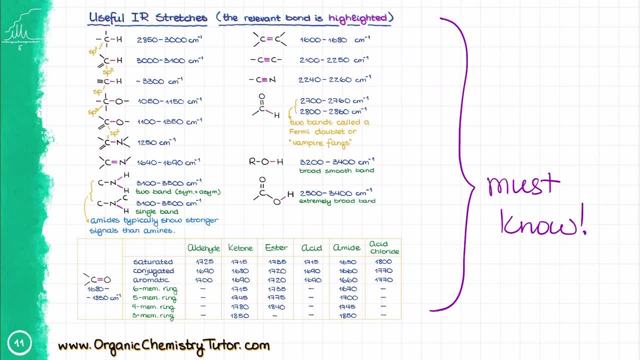 You'll get lost there and you will identify things that are not in your molecule just because you don't know what you're looking for. Beware of the fingerprint and only go there if you really know what to look for. Alright, let's look at a few examples here. Here, I am not seeing anything. 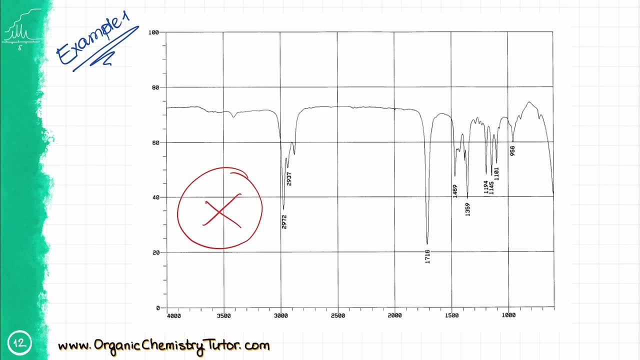 in the 3500 region, so I do not expect any OH or NH groups. Next, I'm seeing these spikes leaning on to 3000 from the right side. This is the indication of the range of the molecule. and this is the indication of the range of the molecule. I think the most likely thing is: 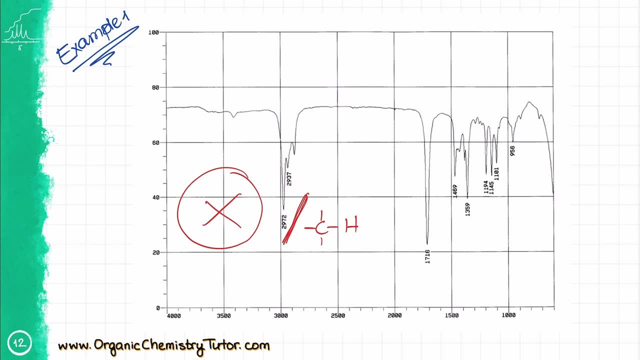 that the molecule is in the range of the carbon hydrogen stretches, and I expect to see those in the majority of our molecules. Then I'm also seeing the carbonyl CO double bond at about 1716 here, which means that we are most likely looking at some sort of a ketone, And 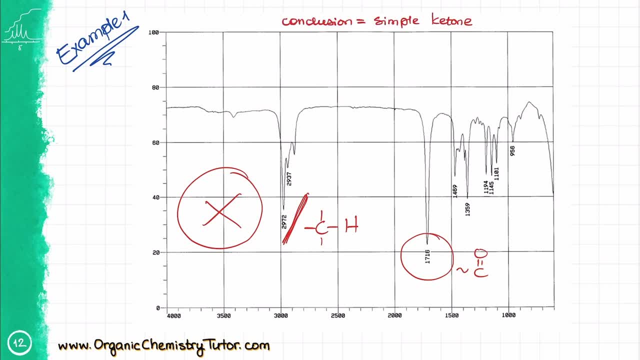 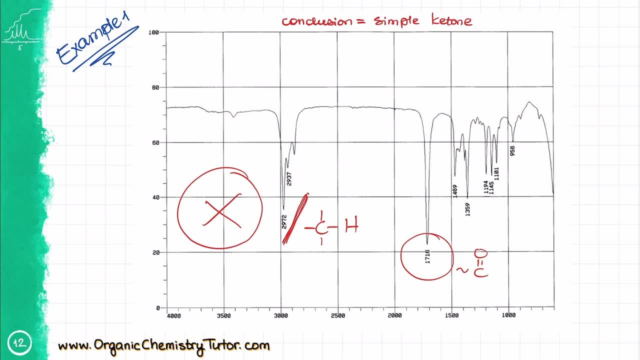 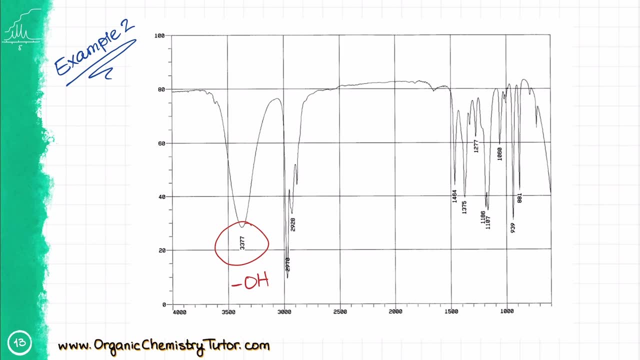 or carbon NMOR, I'd be able to tell you what exactly I'm looking at here. In this molecule, for instance, I have a broad smooth signal at 353300, which is a straight up indication of an alcohol. I'm also seeing some sp3- hybridized carbon hydrogen stretches. 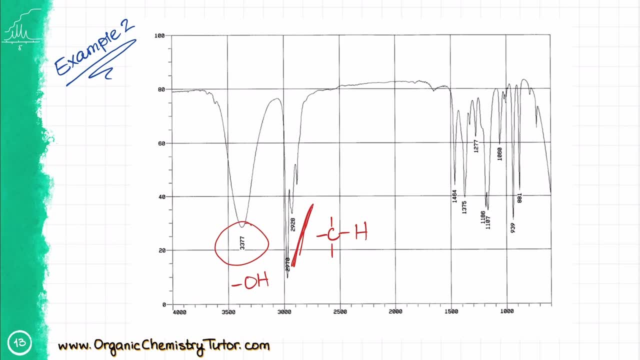 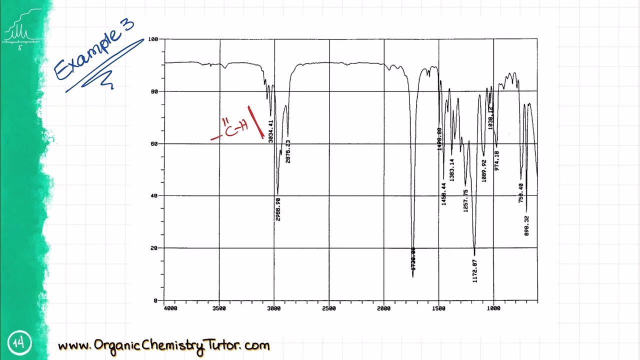 at the right, about 3000 reciprocal centimeters, leaning on it from the right side, and that's about it, Which means that this molecule is most likely some sort of simple alcohol. And here is another example: Here I'm seeing some signals from the sp2- hybridized carbon. 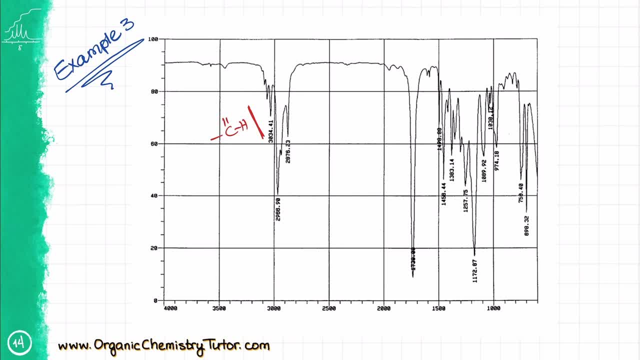 hydrogen stretches, because those signals are a little bit above 3000.. I'm also seeing the typical sp3 hybridized carbon hydrogen stretches, which I would be more surprised if I didn't see, honestly. I'm also seeing a carbonyl at 1730, and there is also a tiny. 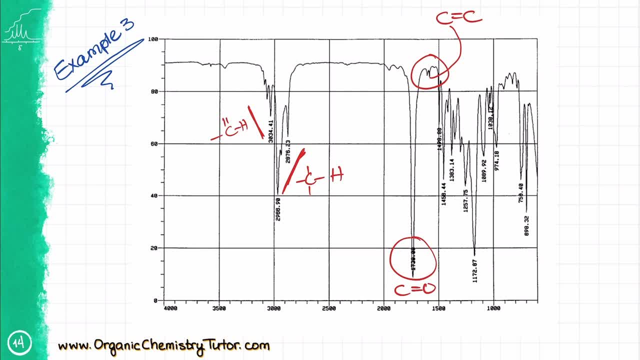 signal over here for the carbon carbon aromatic bond. Looking at the data, we can conclude that this is likely an aromatic ketone or other type of a carbonyl. Looking at the fingerprint region, I can say that this is actually an ester. but I wouldn't expect a typical sophomore organic chemistry student to be able to fish. 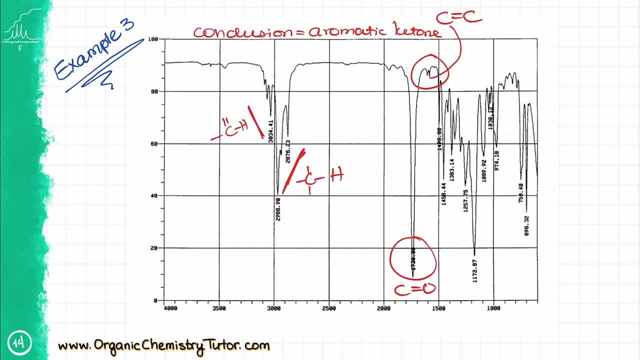 out this information from the IR alone. So normally the IR will be the first step in your spectroscopic determination of a compound, and you'll be able to come up with the complete structure using the combination of the IR, NMR and MMR. 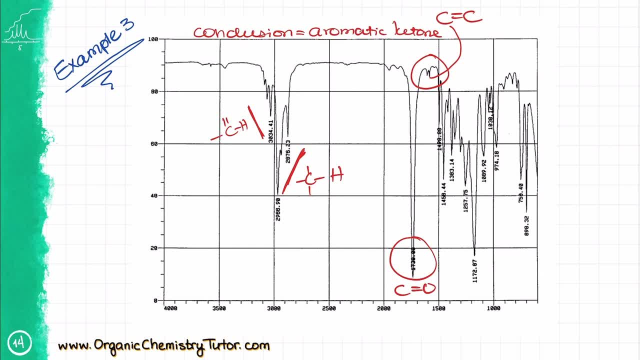 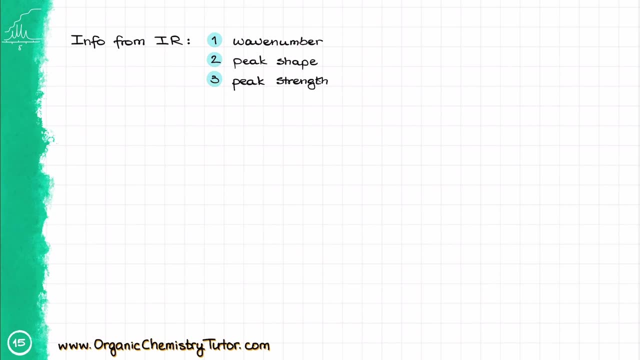 As I've mentioned before, signals can look differently from spectrum to spectrum and from molecule to molecule. so solving spectroscopy questions is a bit of an art, and you can only become good at it if you do a ton of practice. Alright, folks, in these past few minutes we've journeyed through the landscape of the IR. 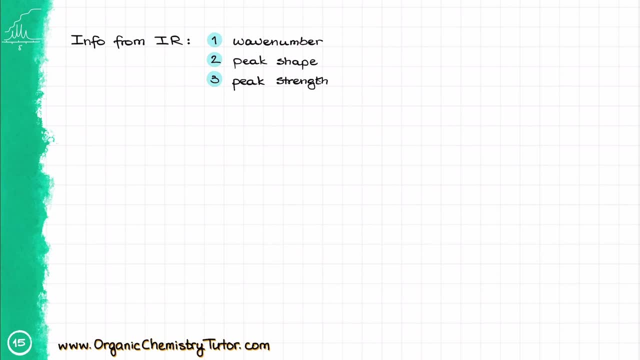 spectroscopy, together, decoding the hieroglyphics of the peaks and valleys on those spectra. You now know how to interpret the wave numbers, The shape of the signals And even their strength. to a certain extent, You've got your reference table, either from me or your textbook or some other place. 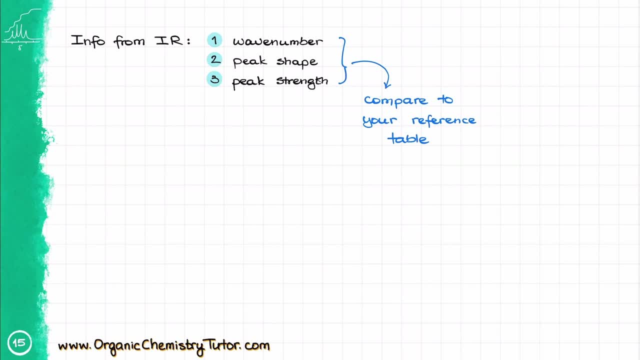 and you've equipped with tips on how to efficiently read the IR spectrum, based on the approach that I outlined in this video. But remember, it's one thing to be a spectator and another to be a player in the field. Your learning curve will only skyrocket when you roll up your sleeves and get down to solving. 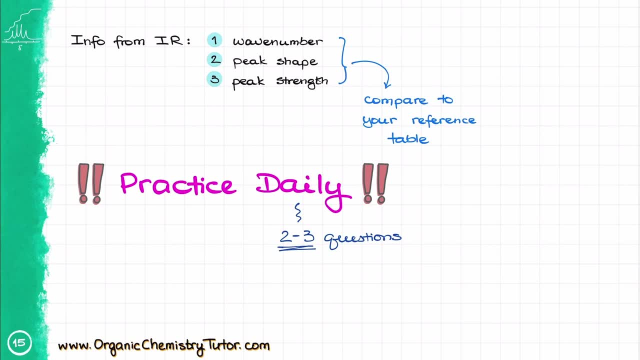 real-world problems. Starting today. take up your time, Solve at least 2-3 spectroscopy problems every single day until your final exam. You'll stumble, you'll scratch your head, you'll get frustrated, but eventually you'll conquer this skill. 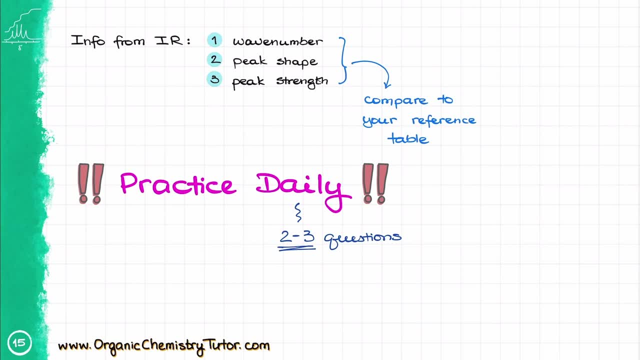 By the time the big test rolls around. you'll handle those spectroscopy questions like a pro. And if you found this video helpful, don't forget to hit that like button and share it with your friends and classmates. Every thumbs up is like a high five to me. 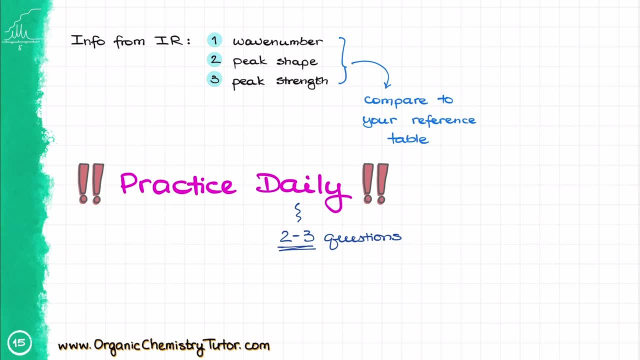 And if you found this video helpful, don't forget to hit that like button and share it with your friends and classmates. If you want more organic chemistry tutorials and solutions, subscribe and hit that notification bell, And if you have questions or need further clarification, drop a comment below. 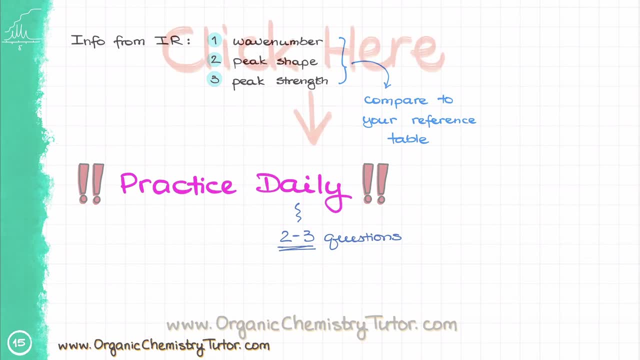 I always love to hear from you guys. Thank you for tuning in. watch this video next and I'll see you tomorrow.